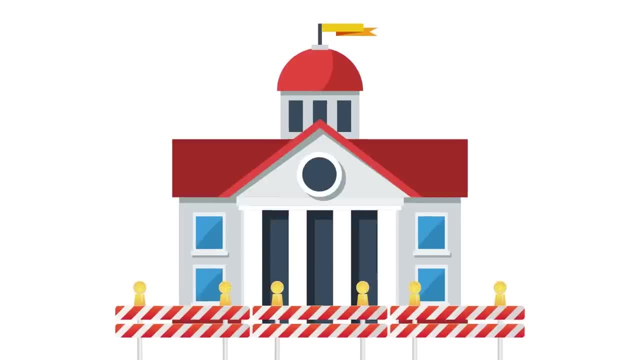 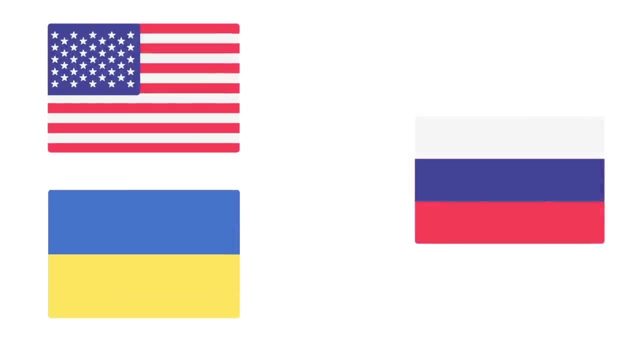 that insecticide. Governments also put in place trade barriers for political reasons or in times of war. In response to the recent Russian invasion of Ukraine, the United States placed sanctions on Russia. A sanction is any action one government takes in order to punish. 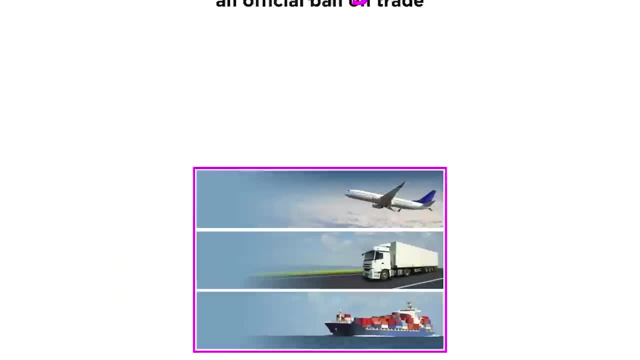 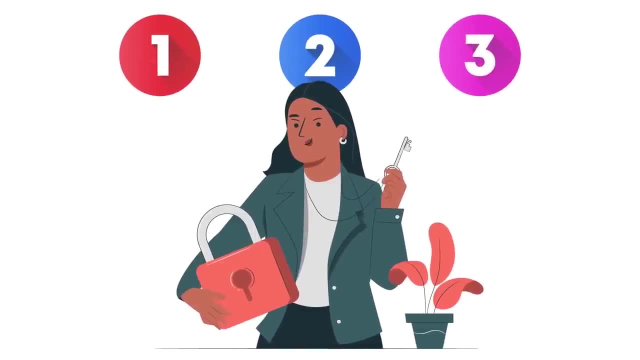 or put pressure on another country. Often that action is an embargo or an official ban on trade. Economists often bring up three potential advantages of a protectionist economic policy. First, protectionism can help workers in industries that might be hurt by foreign. 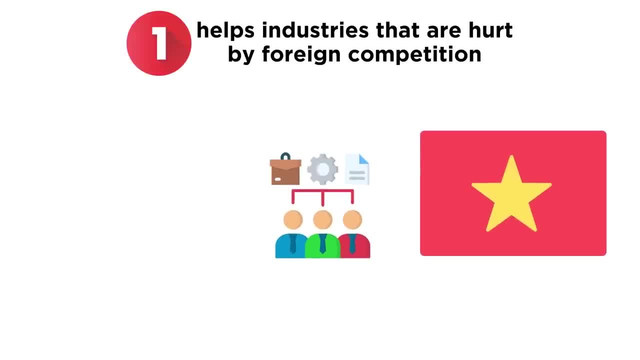 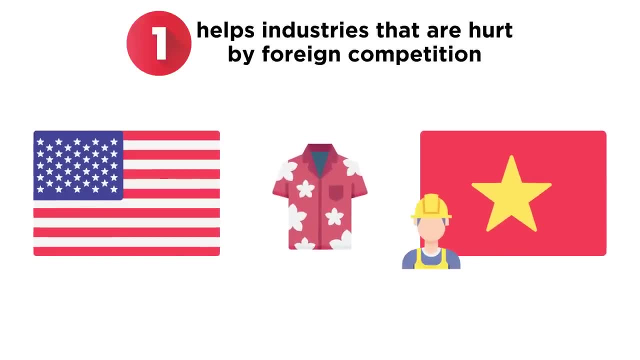 competition Suppose that Vietnam had a comparative advantage over the United States when it came to producing shirts. In particular, workers who made shirts in Vietnam were paid much less than workers who made shirts in the United States, In particular, workers who made shirts in. 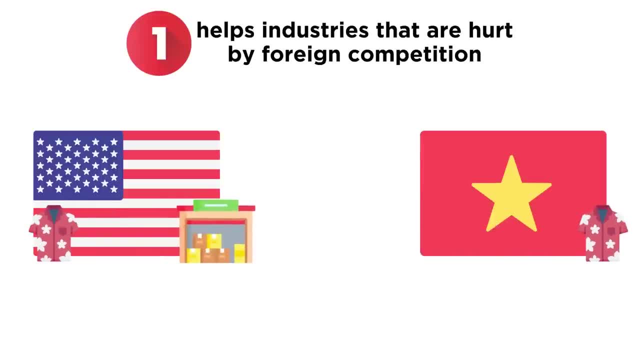 the United States were paid much less than workers who made shirts in the United States. Because of this, American wholesale distributors would have a greater incentive to buy shirts from Vietnam rather than at home in the United States, because it's cheaper. As a result, American shirt companies 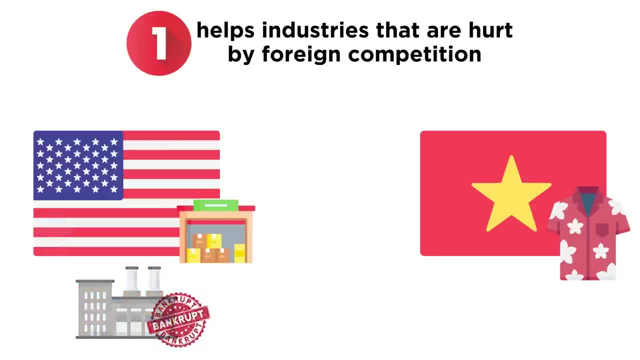 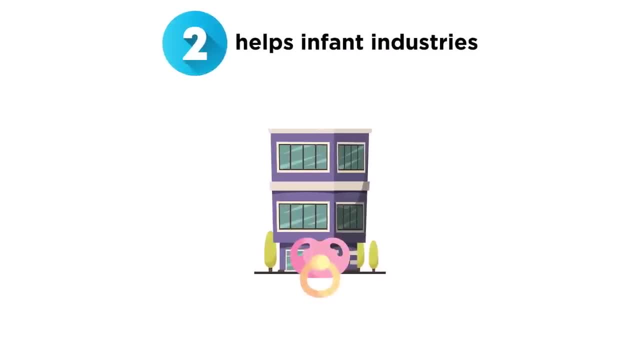 couldn't compete and may have to close their factories and lay off workers. With protectionism, workers are more likely to keep their jobs. Protectionism can also help infant industries or industries that are in early stages of development, Because infant industries are new. 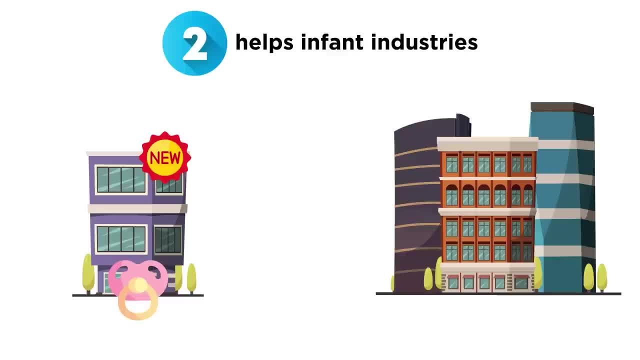 they have a greater chance of losing their jobs and they are more likely to lose their jobs a much harder time competing with more established industries, Because infant industries need time and experience to become efficient producers. tariffs that raise the price of imported goods can provide. 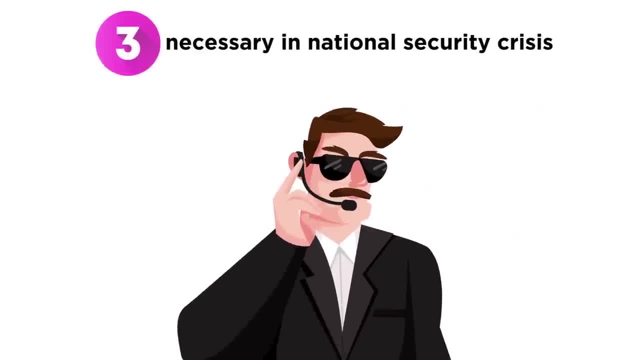 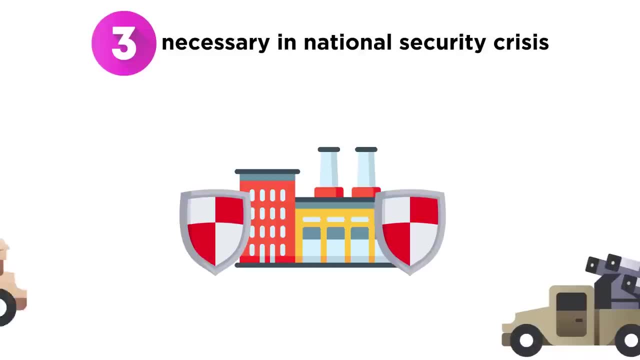 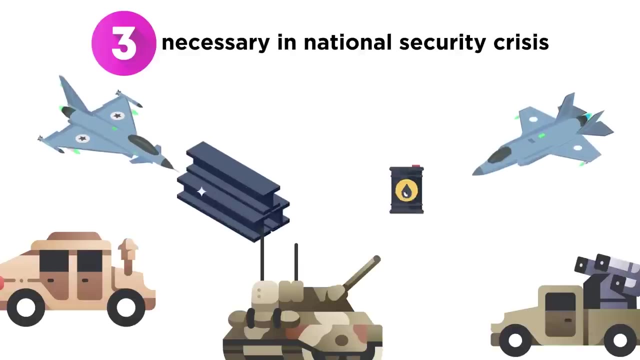 more time until they reach that efficiency. Finally, protectionism may be needed during national security crises. Certain industries may require protection because their products are essential to defending the country. For example, in the event of a war, a country would need an uninterrupted supply of steel and oil. Therefore, domestic production would be prioritized. Ultimately, however, most economists argue that free trade is better than protectionism. First of all, free trade encourages truly competitive markets. If companies are not propped up by governments, they must seek a true comparative advantage and become more. 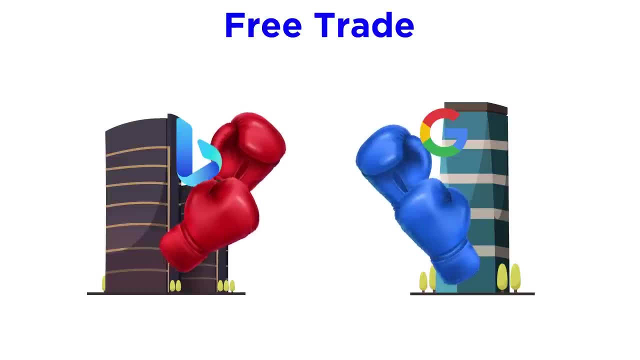 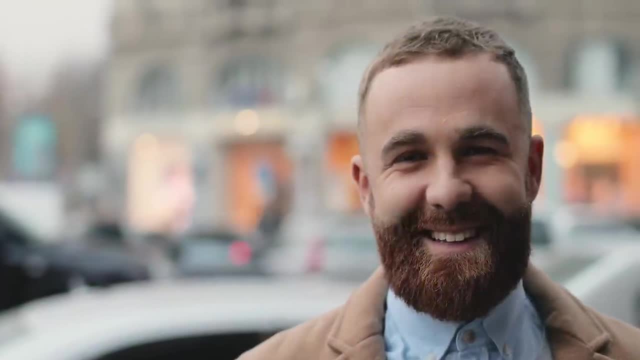 efficient on their own. When companies naturally become more competitive in a free market, they often become more successful. Fundamentally, the biggest winner when it comes to free trade is you, the viewer. You get higher quality goods and services. Perhaps more importantly, you get